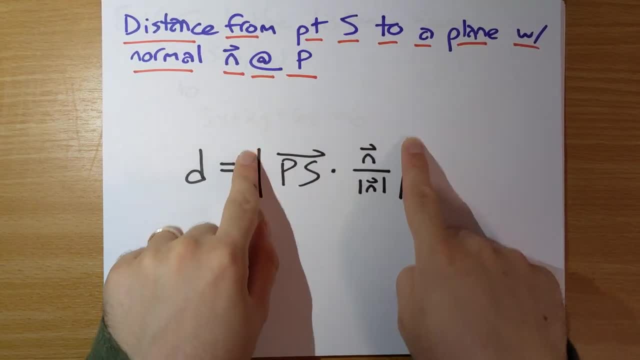 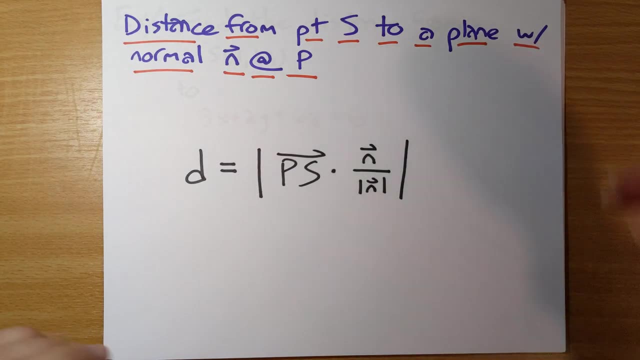 and take. this isn't length, this is absolute value. just to make sure that we don't have that, we don't have a negative length, Just to kind of, you know, I think it's worth drawing a picture here, Just to make sure that we see what's going on. So you know, we have some plane here p. 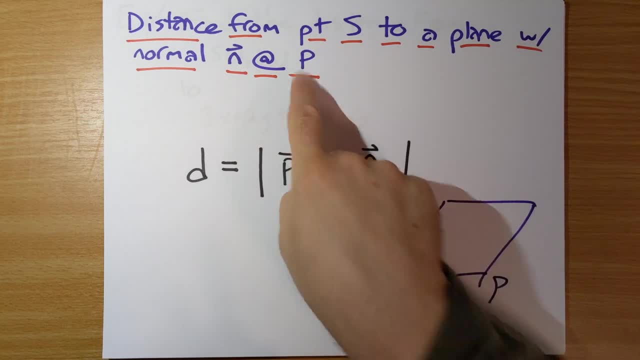 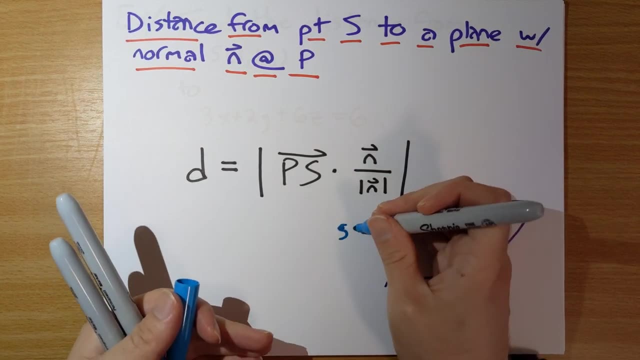 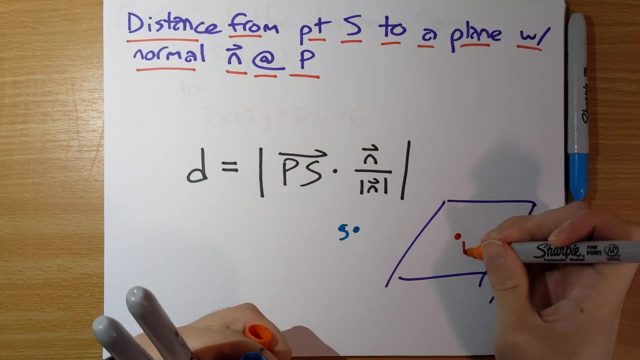 Well, I'll use a scripty p here. This p is actually going to be the point. We have some S point off of the plane. We want to figure out the distance, So we choose a point p on the plane. We can choose any point we want to. 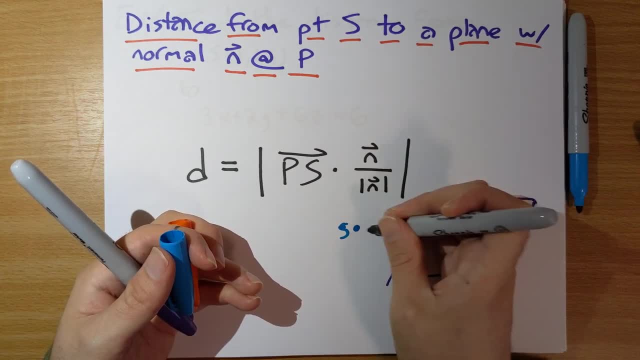 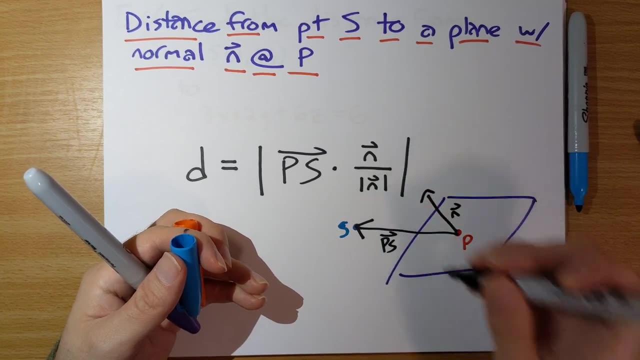 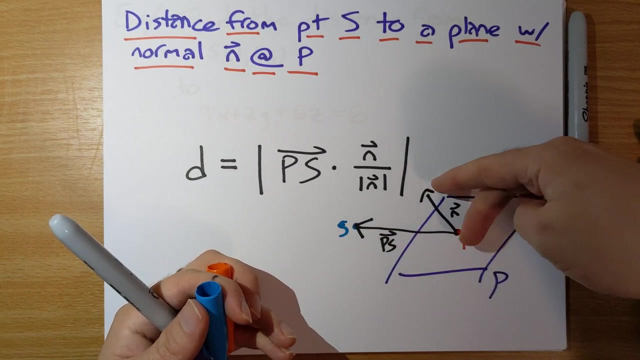 We draw this vector. let's say this is the normal vector here. This is p S, so u p S the the vector from p to S here. dot product with the normal vector. let me you know that's a normal. 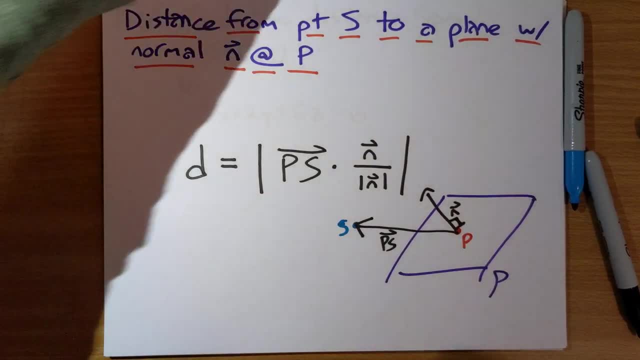 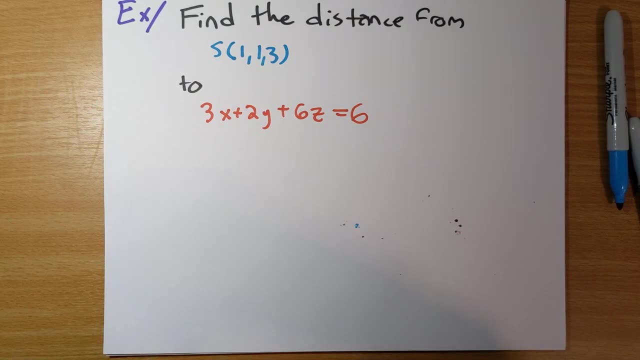 vector That's been scaled appropriately, so it's a unit normal vector. Okay, so let's go ahead and ahead and get into an example of this. So find the distance from the point 1,, 1,, 3, that's our s. 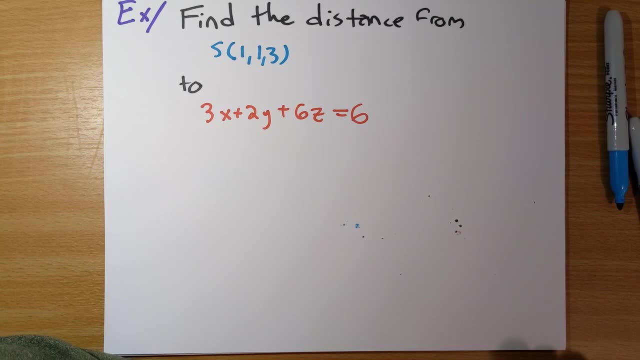 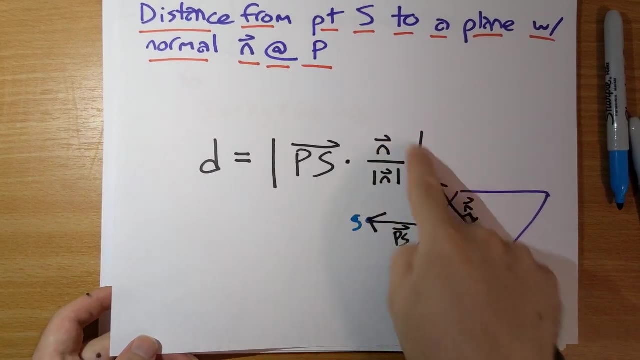 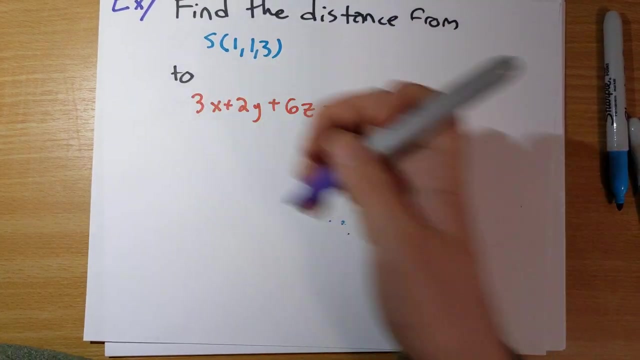 to the plane: 3x plus 2y plus 6z is equal to 6.. So first off, let's realize that we need a normal vector. And so how do we find a normal vector? We can get n by simply taking the coefficients. 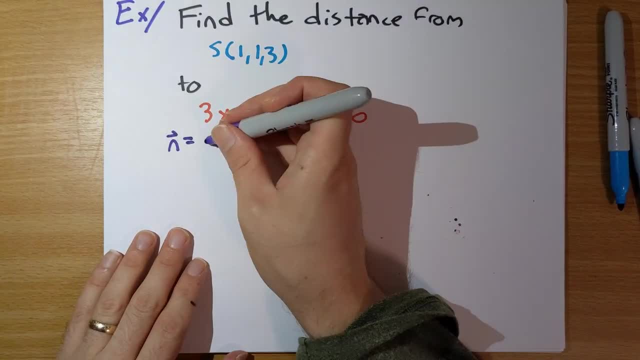 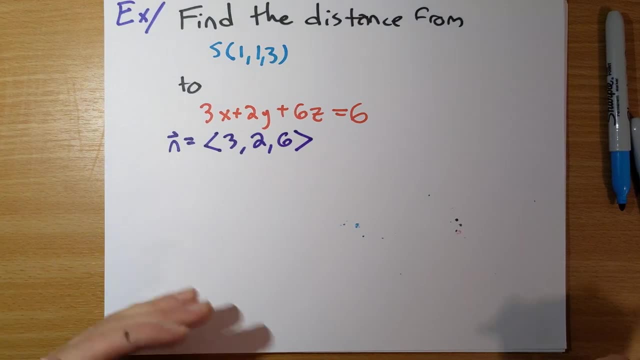 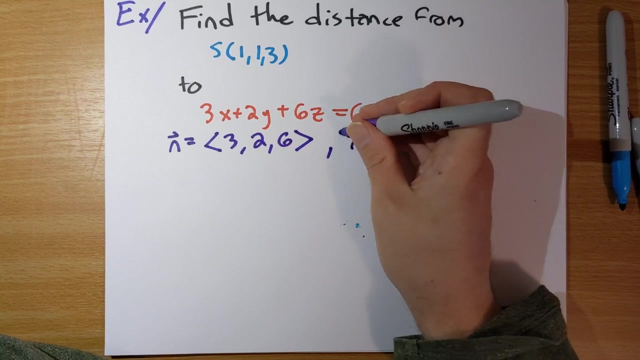 of x, y and z respectively. So 3,, 2,, 6.. This is our normal vector. Well, we also need to find the length, the magnitude of the normal vector. So the length here is going to be the. 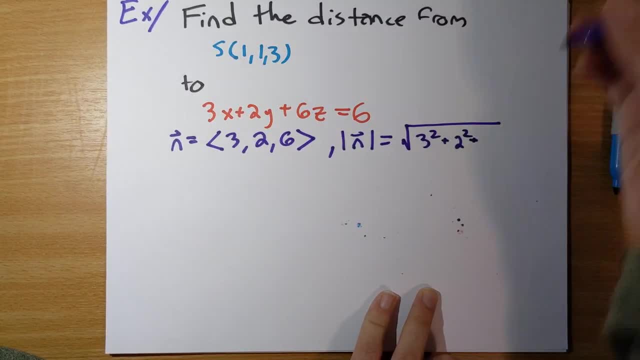 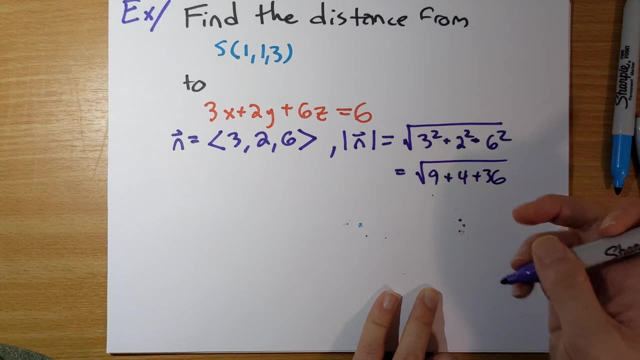 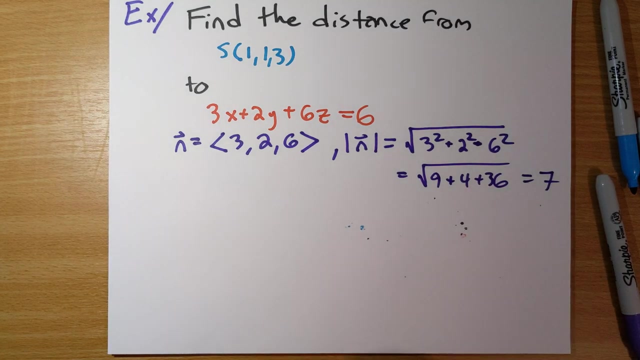 square root of 3 squared plus 2 squared plus 6 squared And that's going to be 9 plus 4 plus 36, that's 49 under the square root. so the length here is 7.. Okay, we need okay. 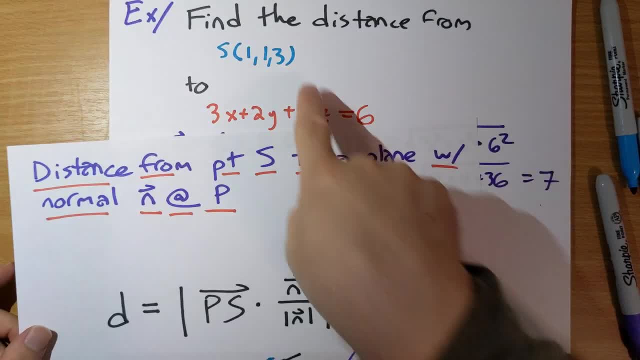 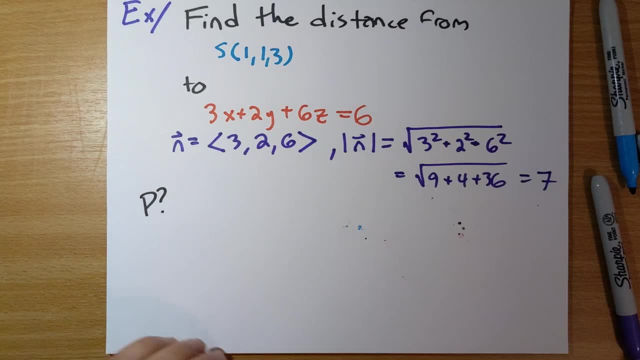 so we have our normal vector, we have our length, we have our point S as given to us in the problem. Now, the thing is that we need a point And we can choose any point that we want to. we can choose any point that we want to for our purposes here, Probably. 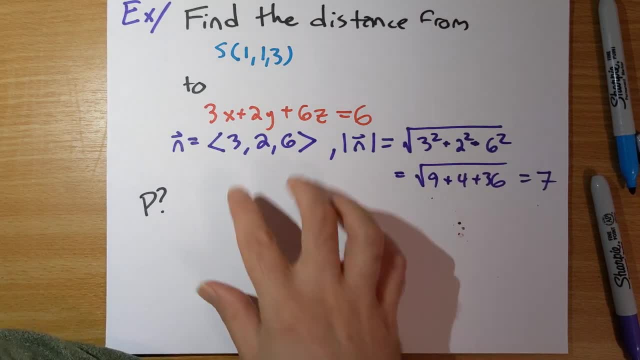 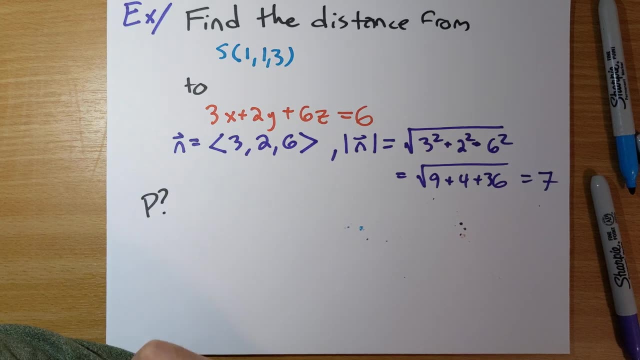 the easiest way to do this is to find an intercept, So that would be: set a couple of: set X and Y to zero and figure out what Z has to be set X and Z to be zero. figure out what Y has to be set Y and Z to be zero and figure out what X has to be. Let's have X, let's. 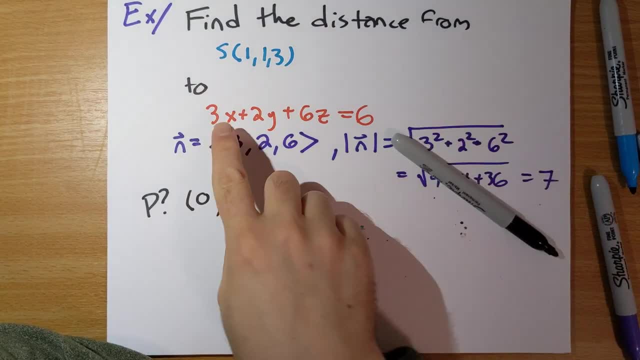 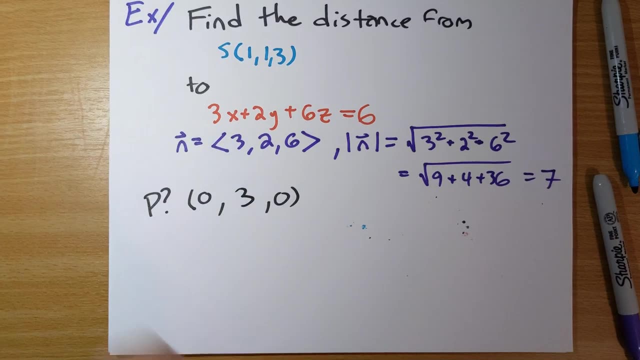 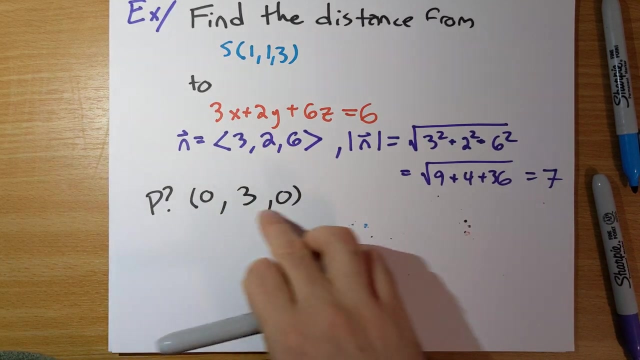 have Z and Z be zero. If X is zero and Z is zero, our equation is: 2Y is equal to 6.. And so our point here is 0,, 3,, 0.. Okay, so if we're using this as P, we want a vector. 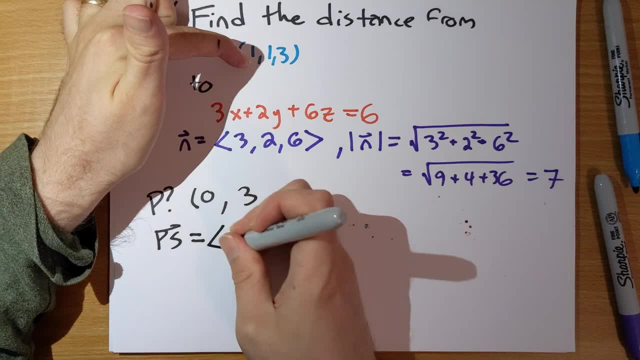 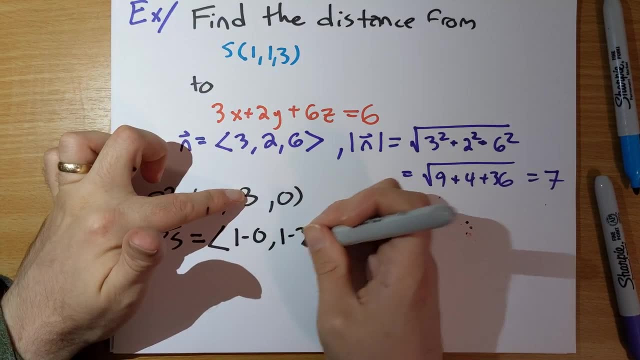 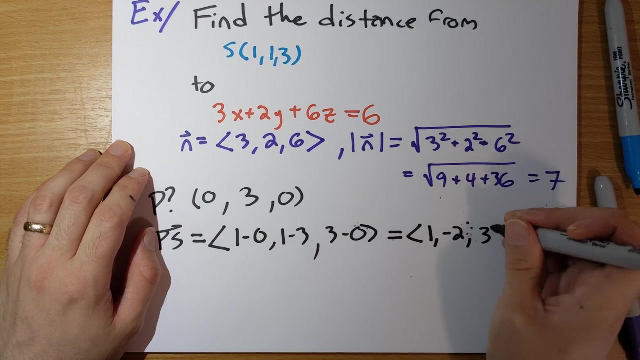 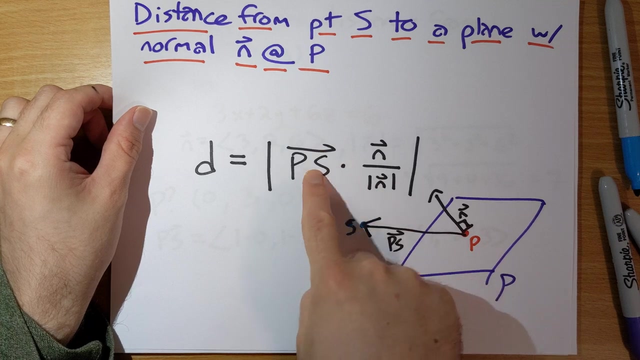 from P to S, and so that would be 1 minus zero, 1 minus 3,, 3 minus zero, So that is 1, negative 2 and 3.. And so now, using the formula, it's just going to be the dot product of our PS vector with. 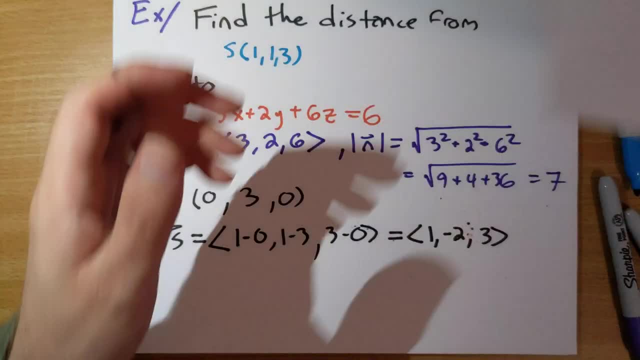 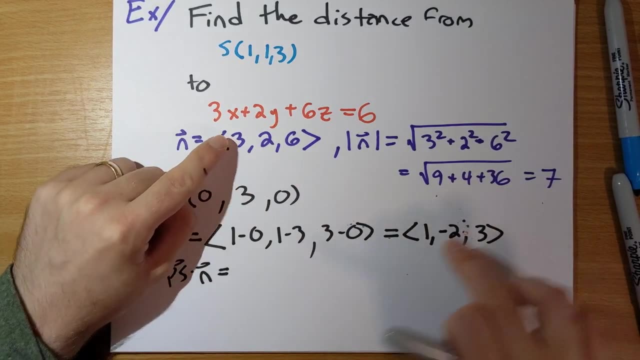 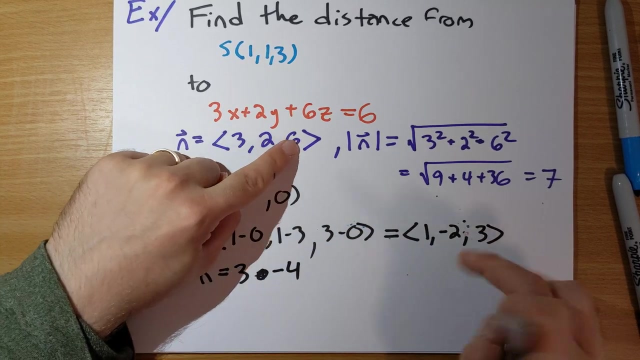 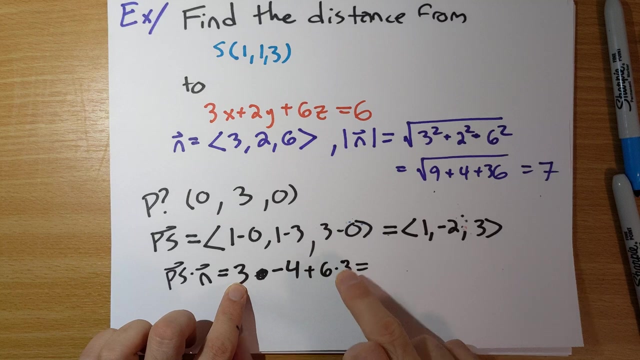 a normal vector divided by the length of N. So PS dot product N is going to be a dot product of this. with this will be the X squaredações: 3 times 1,, 2 times negative 2, and 6 times 3 is 18.. So that would be 18 plus 3 is 21. 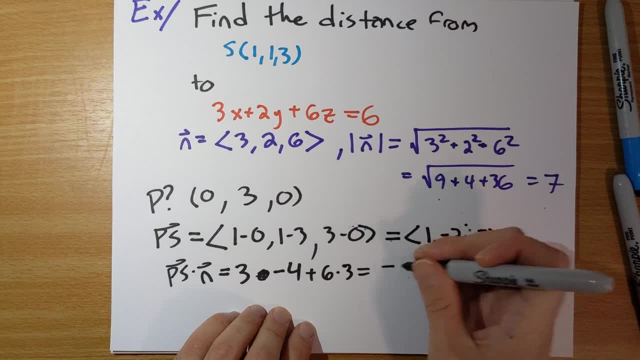 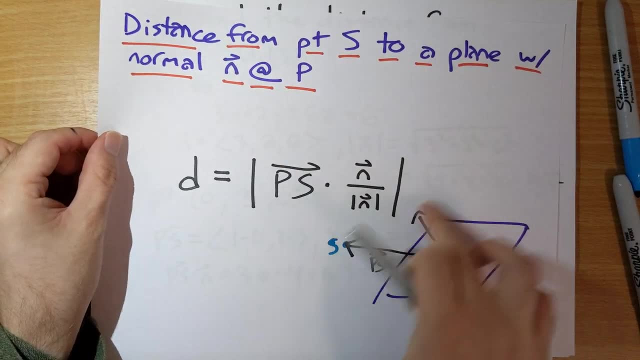 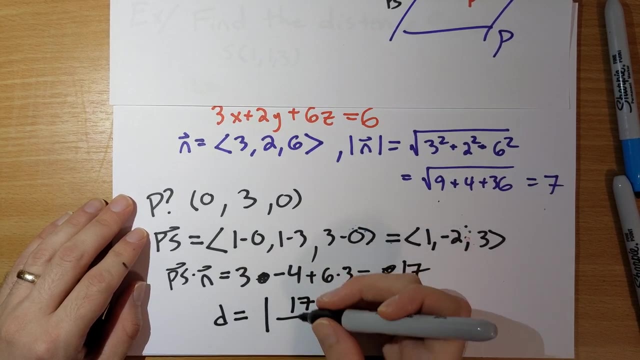 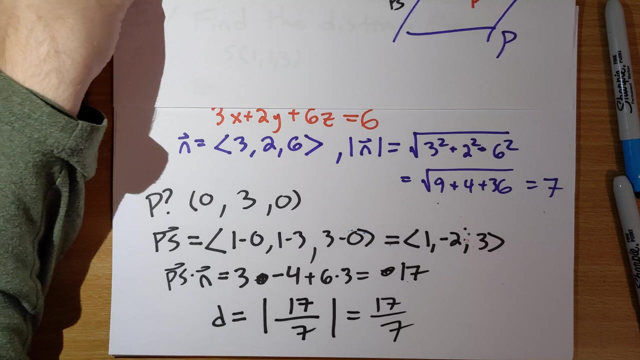 minus 4 is 17.. Okay, and so then our distance here is going to be 17 divided by 7.. Absolute value of that: everything inside is positive. so we just have 17 over 7.. I should point out that. 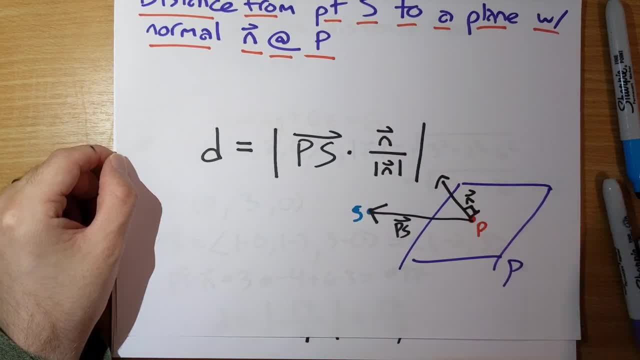 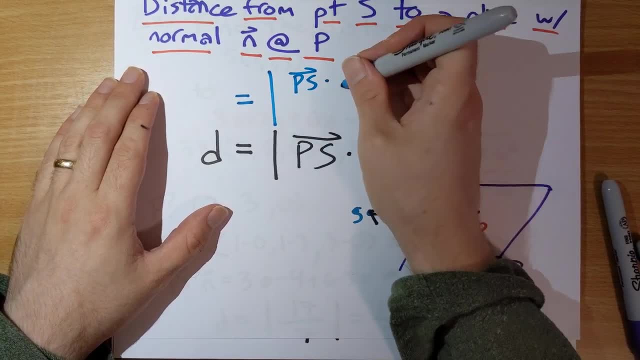 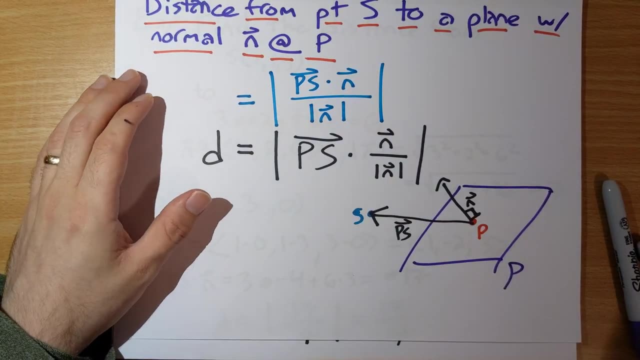 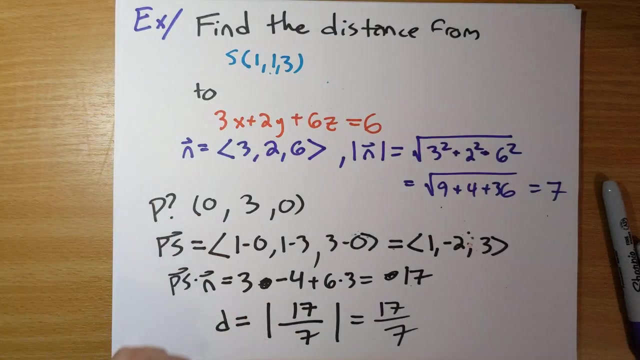 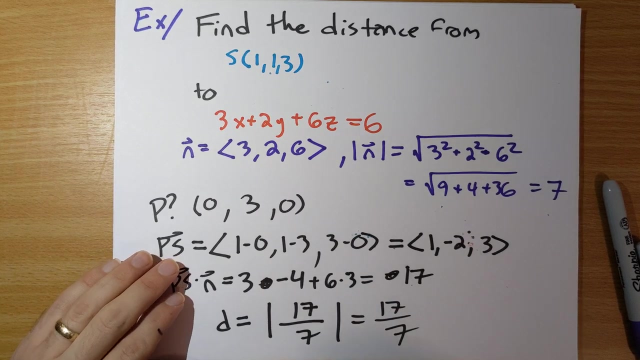 computed it was. I did the PS vector, dot product, the normal vector, and then I divided by the magnitude of the normal vector. These two are equal to each other by dot product properties. I said it doesn't matter what point that we choose here. I think maybe it would be in. 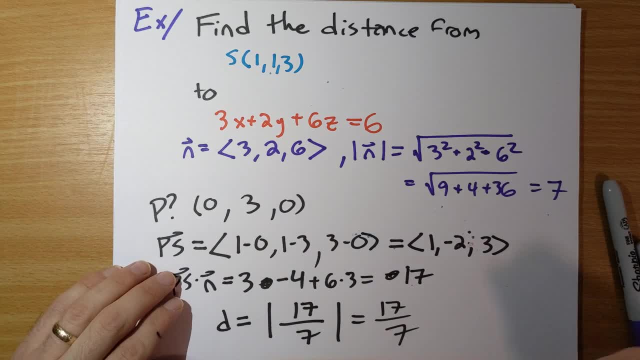 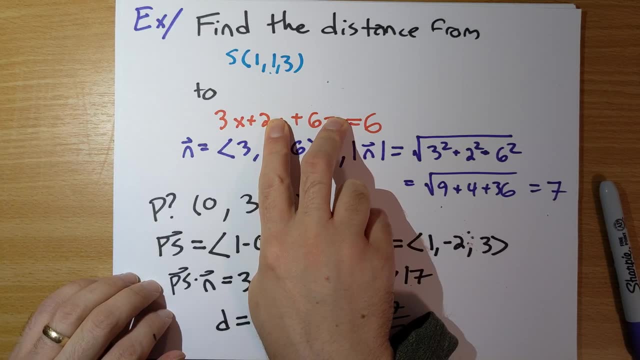 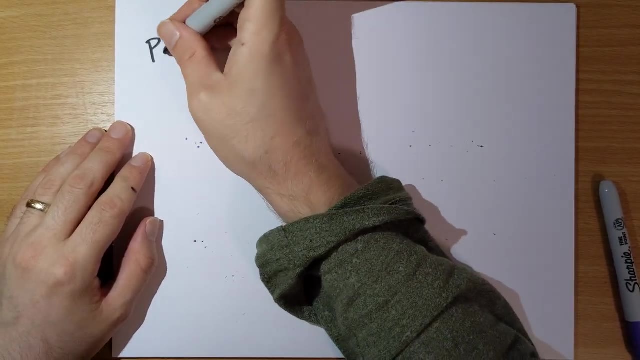 this directive. Let's just choose a different point. If we set y and z to be 0,, we would have 3x is equal to 6, and so that would be x is equal to 2.. So if instead let me call it q, here is the. 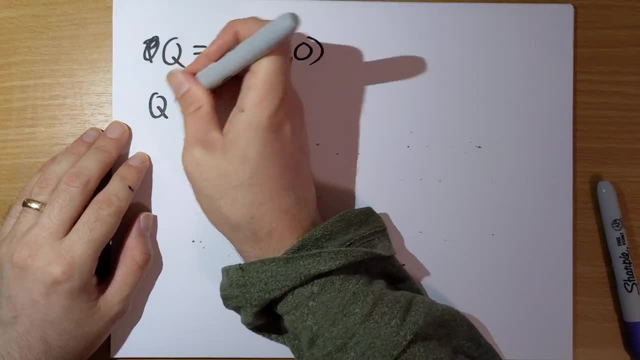 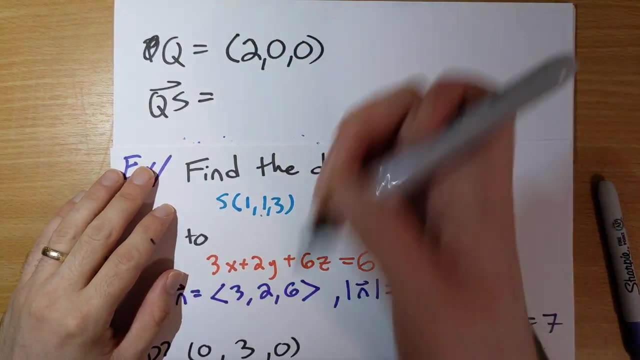 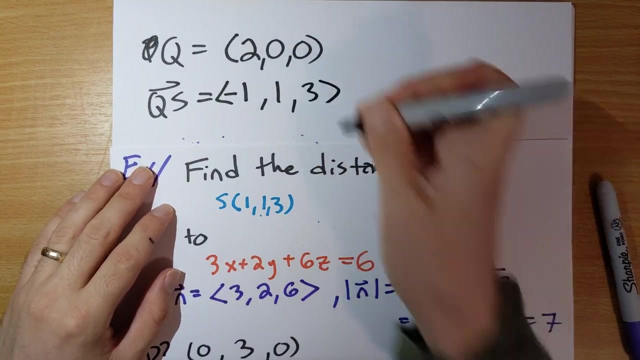 point 2, 0, 0.. So vector from q to s, where s is 1,, 1,, 3.. 3 would be: 1 minus 2 is negative, 1.. 1 minus 0 is 1.. 3 minus 0 is 3.. And so everything works out. 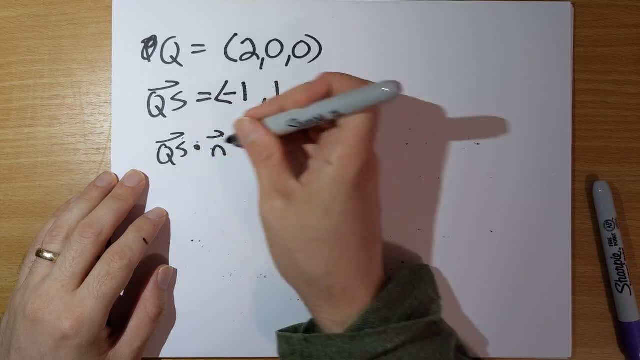 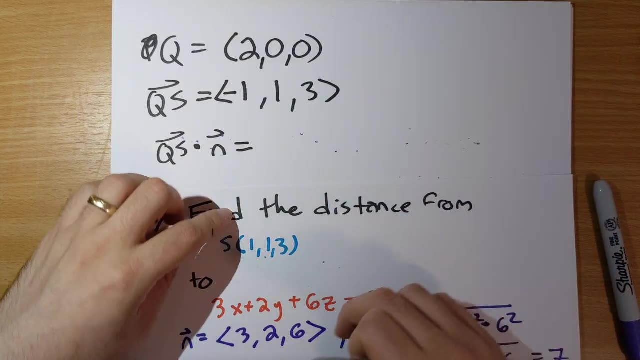 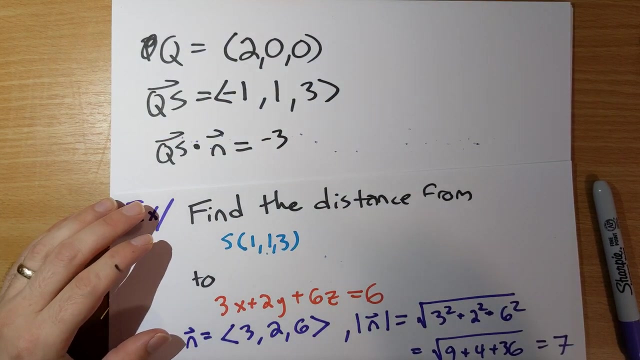 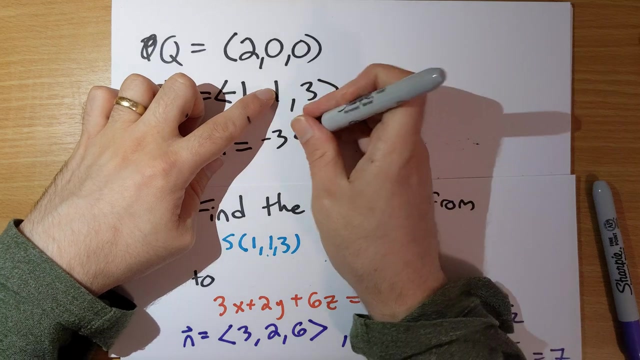 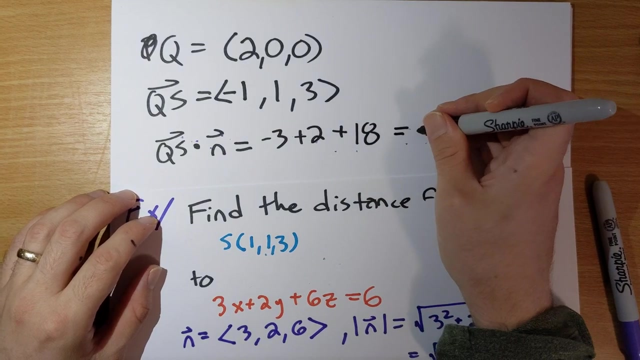 well, qs dot product n, where n here is 3,, 2, 6.. This would be 3 times negative: 1 is negative, 3.. Let's see So: 3 times negative, 1 is negative 3.. 2 times 1 is plus, 2.. 3 times 6 is 18.. Once again, 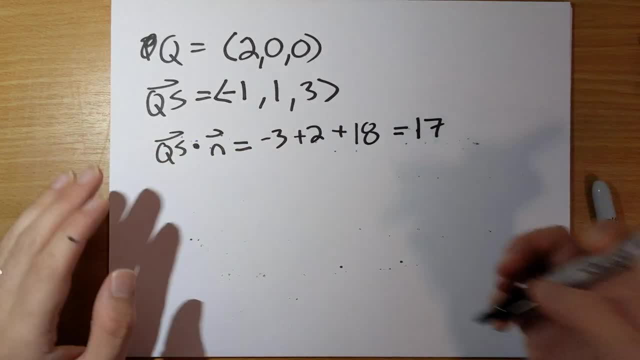 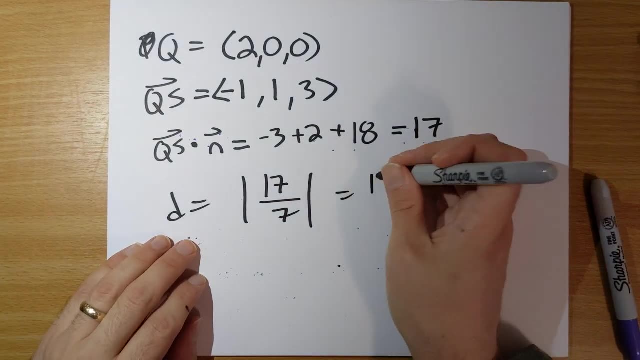 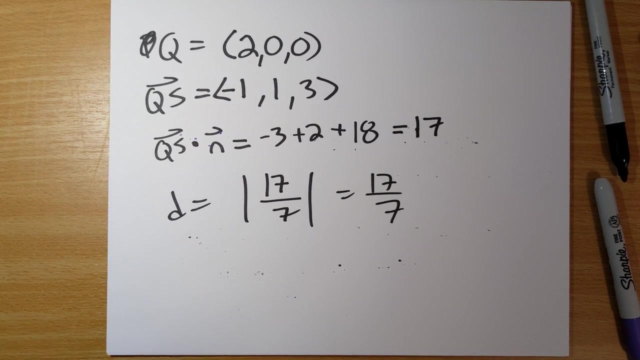 this ends up as 17 for our dot product here, And so the distance would be absolute value of 17 over 7, which again is 17 over 7.. So it genuinely does not matter which point you choose on the plane. If you crunch through everything, you'll get the correct answer.